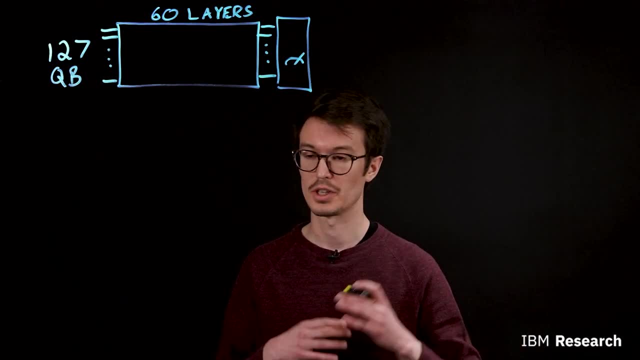 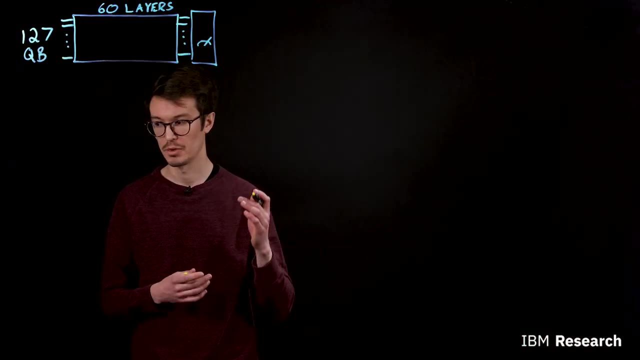 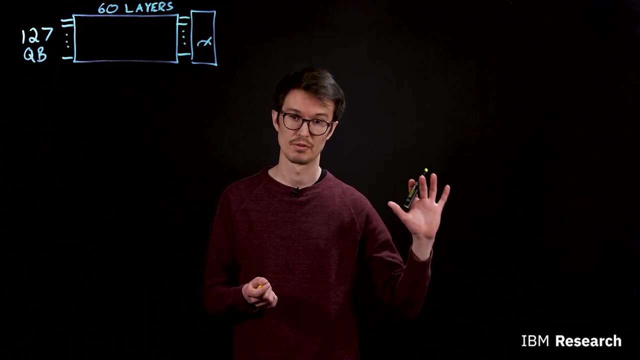 they have some noise. in the hardware, we're still able to extract useful results, or reliable results using a class of techniques known as quantum error mitigation, And so this is giving us a space to start exploring what we can do with these devices, even before the era of fault tolerance in long-term quantum computing. 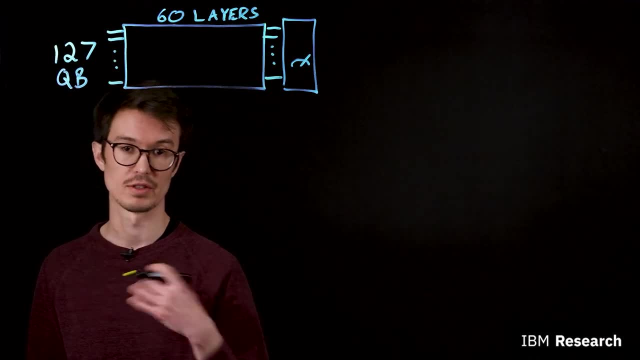 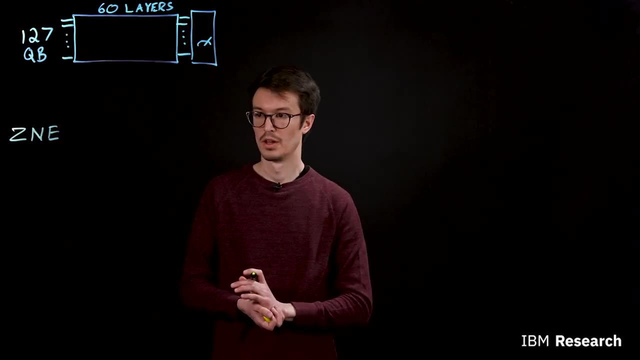 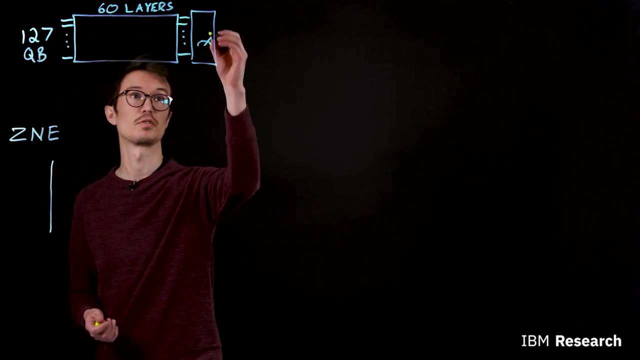 And in particular in this experiment we used a technique known as zero-noise extrapolation or ZNE. So how does ZNE work? First we'll run our circuit and get some estimate of our observable. Say we want to learn some observable property O. 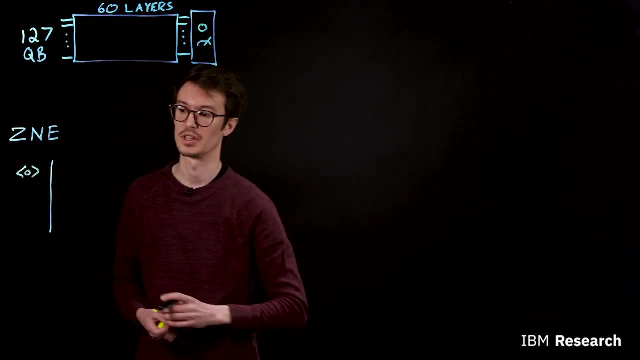 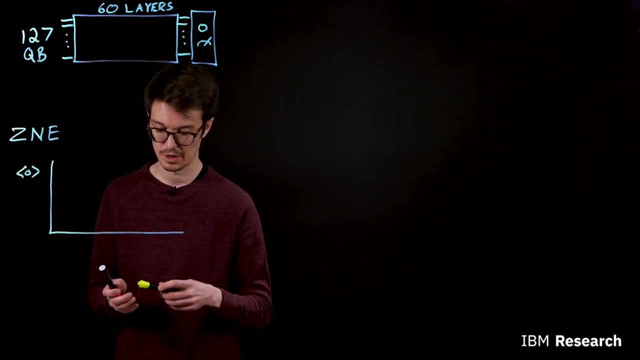 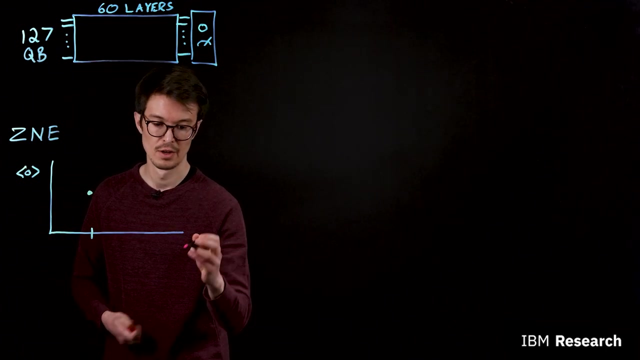 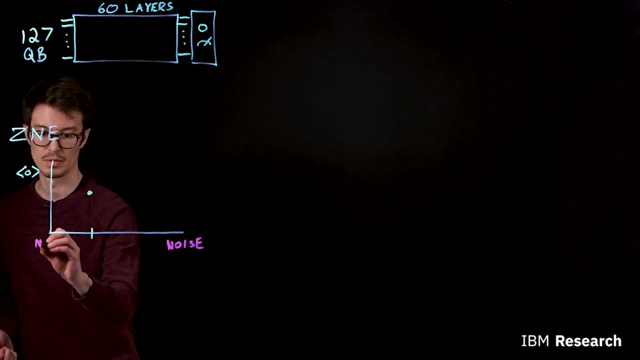 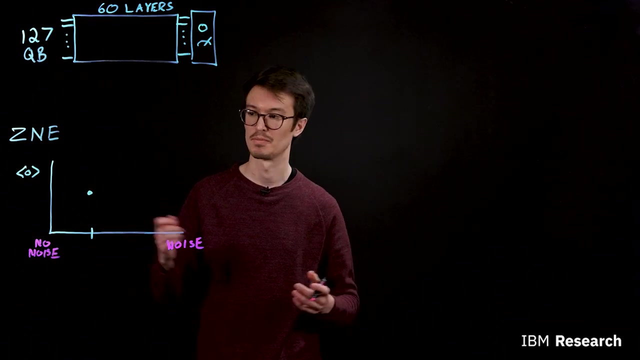 And we want to look at particular at the average or expectation value of that, that property. We run our experiment and we get some result. However, this result may be made inaccurate by the presence of noise on the quantum hardware. Ideally, we'd like to get an estimate of what the answer would be if we ran this, if we solved this problem without any noise. 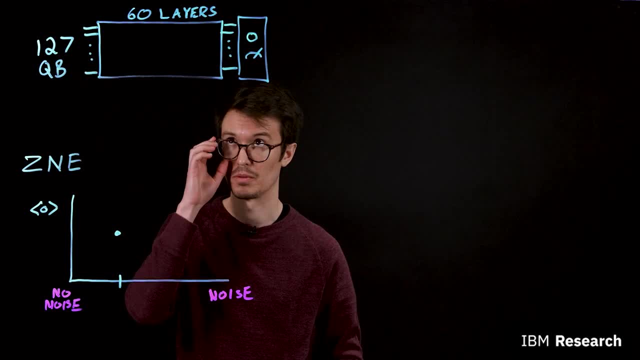 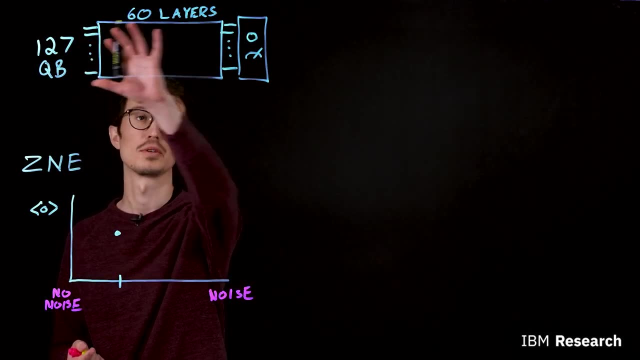 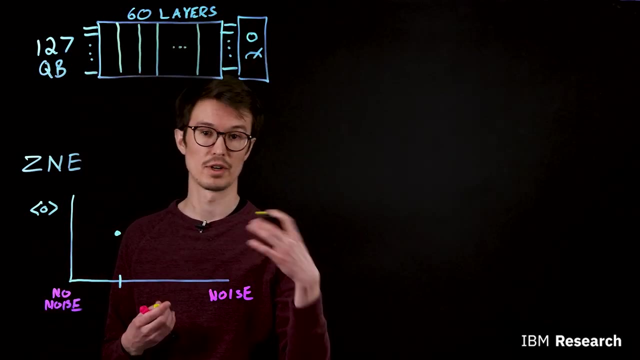 So how do we correct for the inaccuracy brought about by the noise on the hardware? Well, first we'll get to the second tip: go and learn what the noise is actually doing, how it's behaving on the device. So we'll take the problem that we're studying, we'll break it up into layers and then for 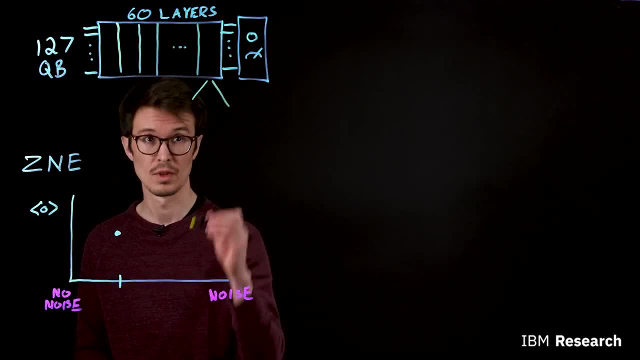 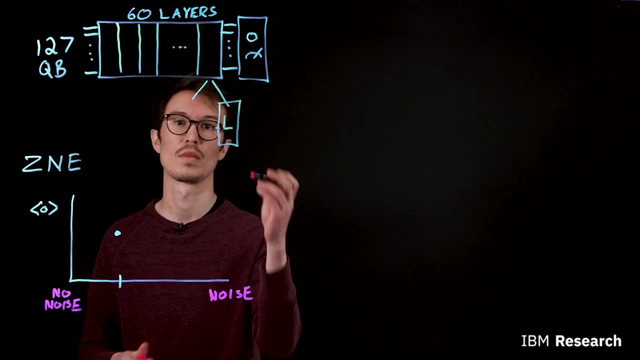 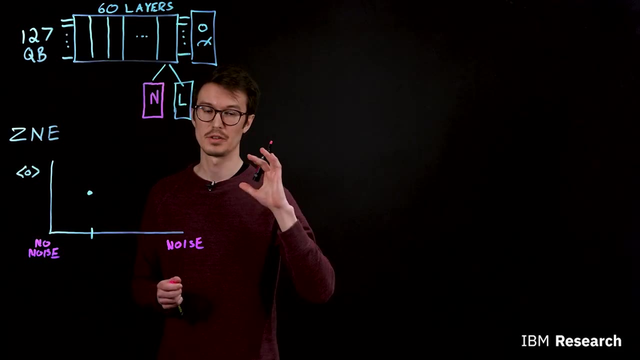 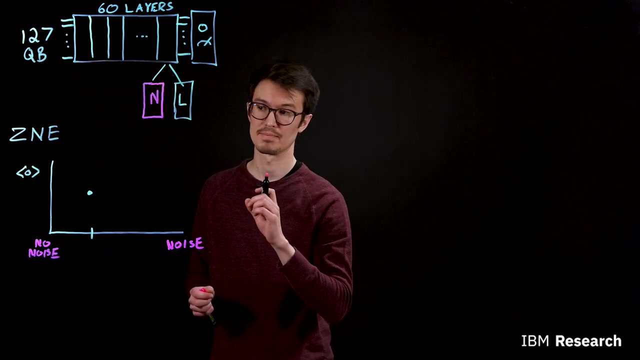 each layer. we'll further decompose that into two pieces, One that captures the ideal behavior of that layer and another representing the noise, And so by doing a bit of extra additional work, we can go and measure how all of these noise pieces in the circuit are behaving. 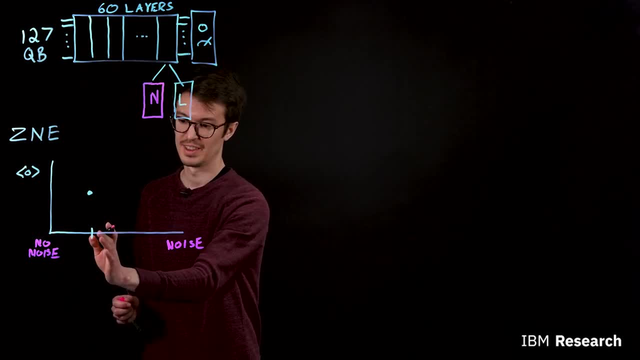 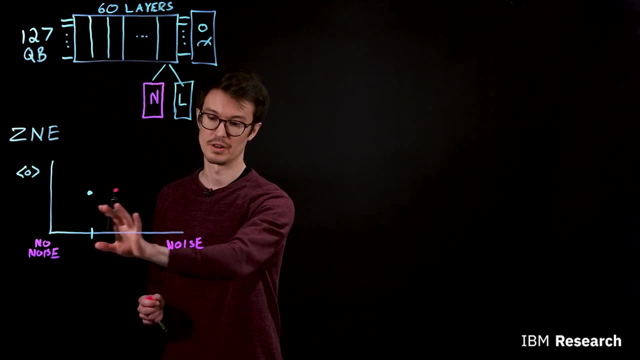 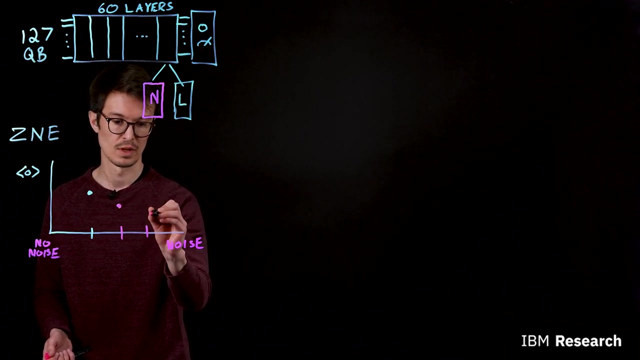 And once we have that information, although it's hard to turn down the level of noise that's happening on the hardware, we are able to use that knowledge to turn it up. So by repeating the experiment in the condition where we've ended up with a noise piece, we're able to turn it up. 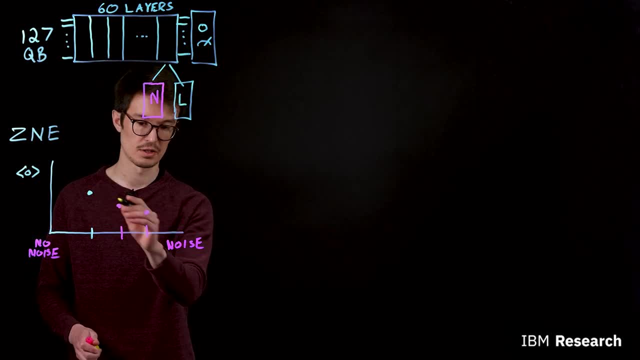 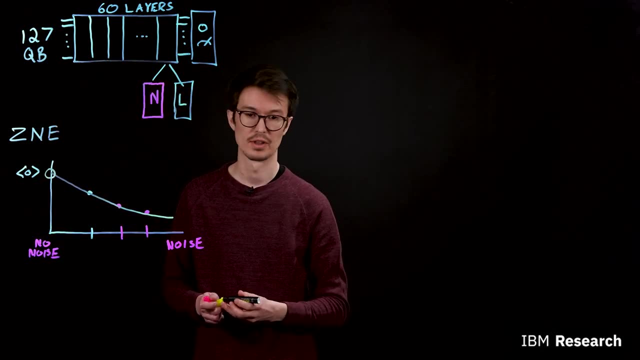 So by repeating the experiment in the condition where we've ended up with a noise piece- increase the noise- we can then get additional results which we can use to extrapolate back and estimate the true value in the case of no noise on the hardware. 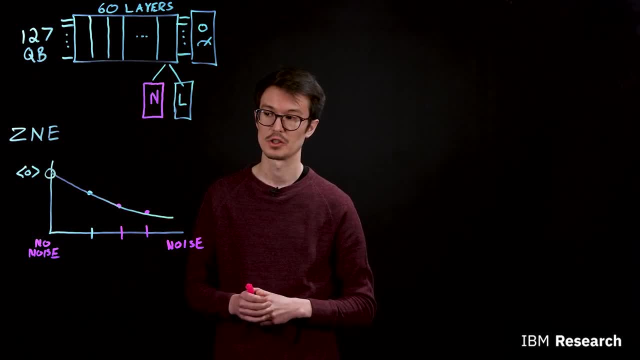 So that's a bit about the basic theory underlying our experiment And with that out of the way, I'll pass things over to my colleague and co-author to further explain details of the experiment. Thanks, Andrew. My name is Yongseok Kim, researcher from IBM Quantum. 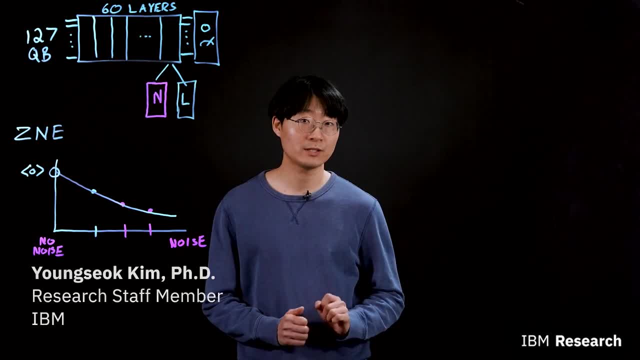 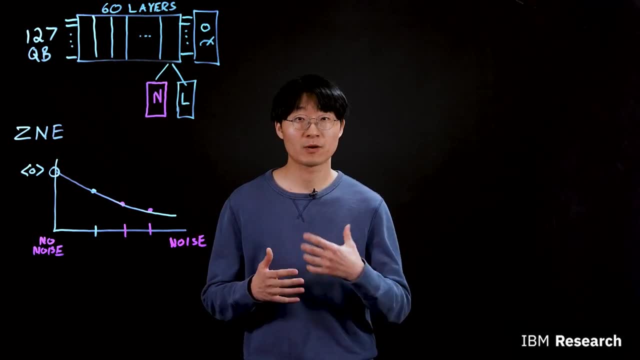 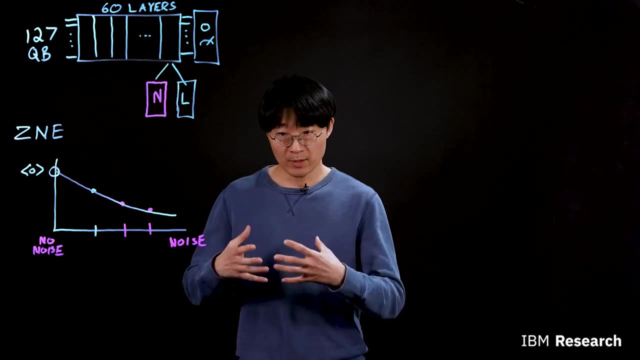 Like what Andrew said, I'm going to talk about a little bit more detail about what we did. So, to make a long story short, what we did is we performed an experiment on spin dynamics of transverse field easing model, So we performed an experiment on our quantum processor. 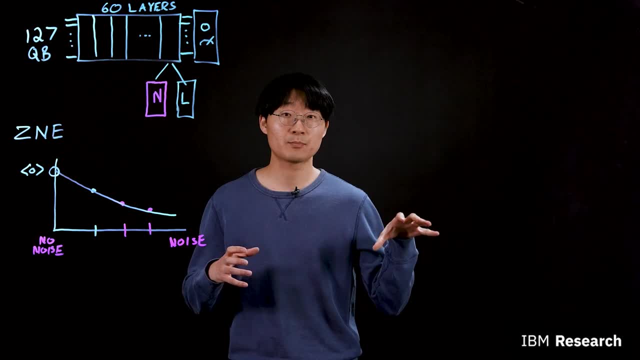 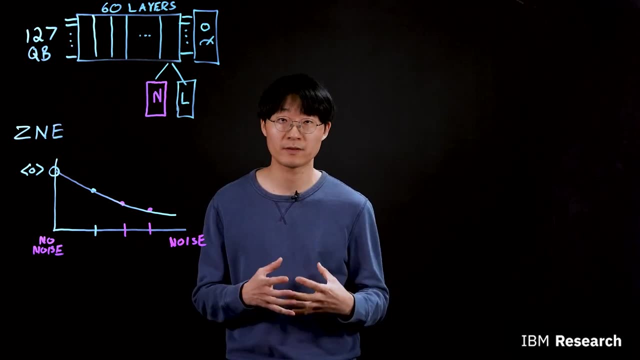 and we worked with our collaborators at UC Berkeley and they produced corresponding results in a classical computer And we compared our results against each other to build the confidence that we had. And that's what we're going to talk about today. So let's take a look at some of the experiments on our method. 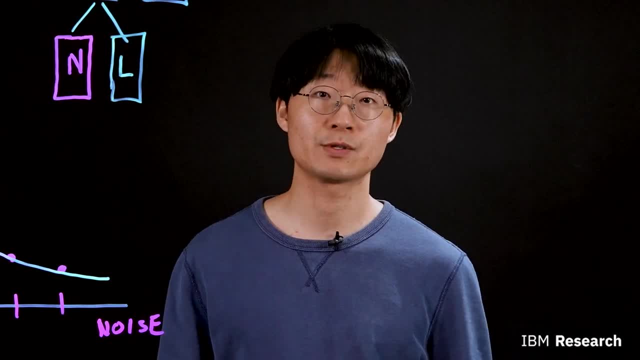 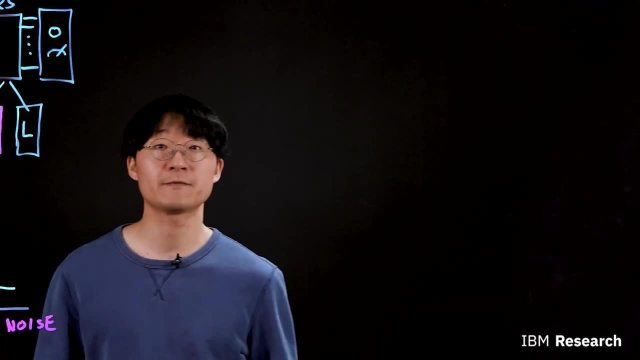 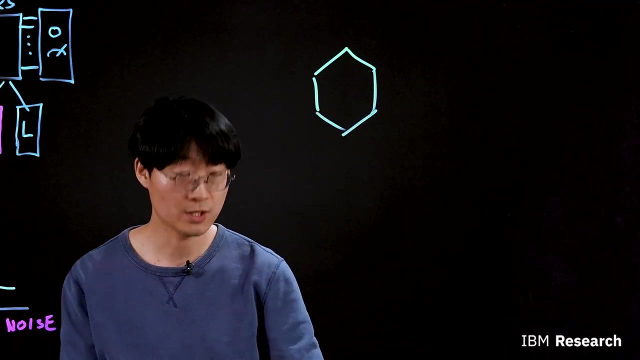 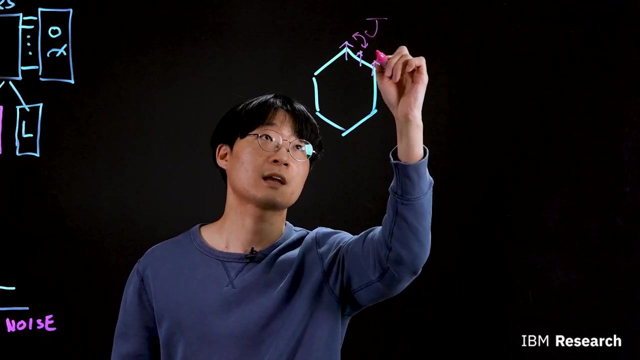 So we use ZNE as our error mitigation method. We use an IBM KEY 127 qubit processor to study the spin dynamics. To be more specific, we map our spin lattice to our hardware topology, which is heavy X topology, And this spin is governed by nearest neighbor interaction, J and. 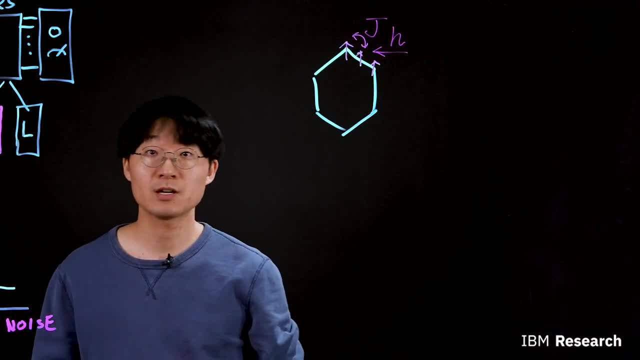 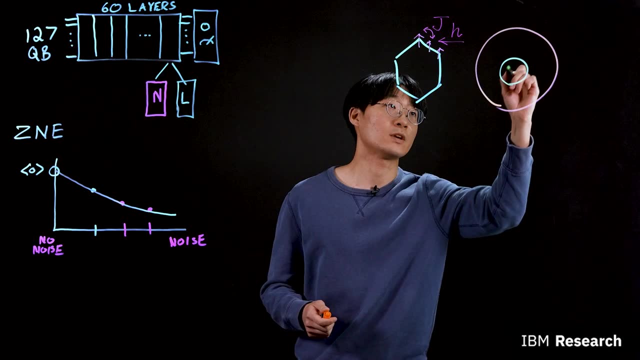 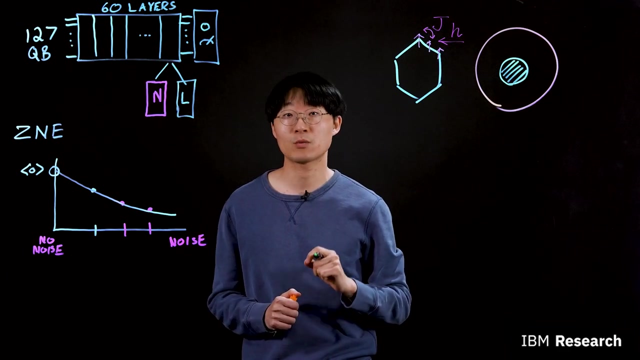 global transverse field H. So let's take a look. So, as you can see, here we have large parameter space to explore, And among this parameter space we have some parameter that results in Klippor circuit, Meaning we can efficiently simulate this circuit. thereby we obtain ideal value. 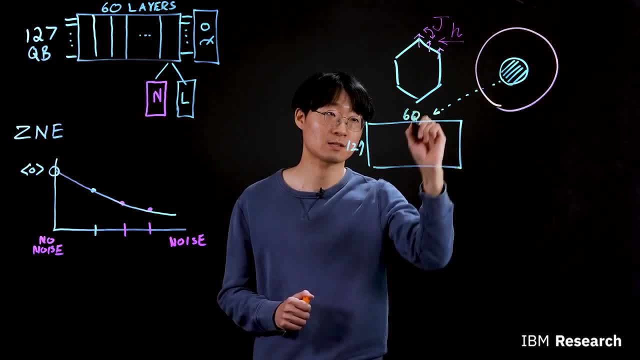 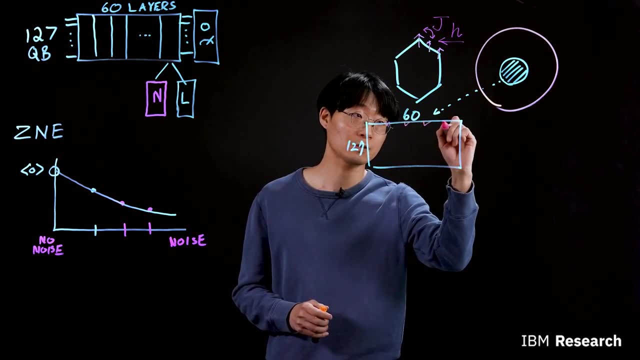 So we utilize this nice property to examine our results. So here is the circuit: 127 qubit and depth of 60.. Two qubit gates Along the way we check our results from HONON computer, and that agrees well with each other. 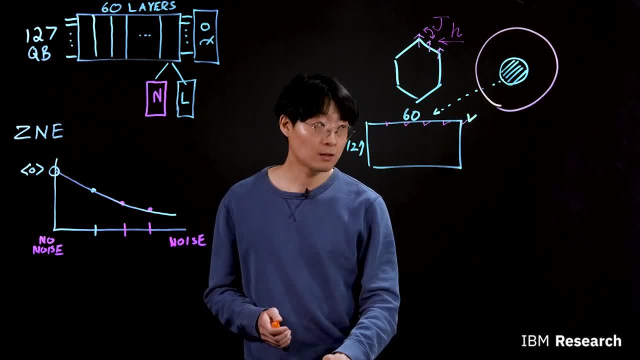 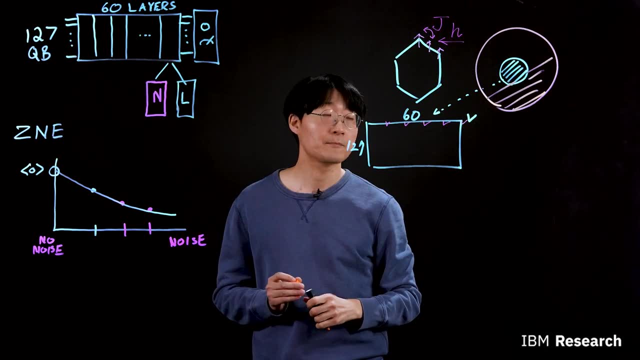 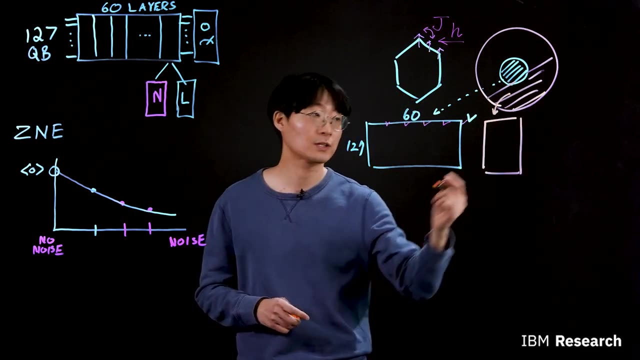 So there's one check. Of course, there are large parameter space which results in non-Clieffer circuit, which is in general hard to verify. Instead, what we did is we take the parameter that results in non-Clieffer circuit, we go. 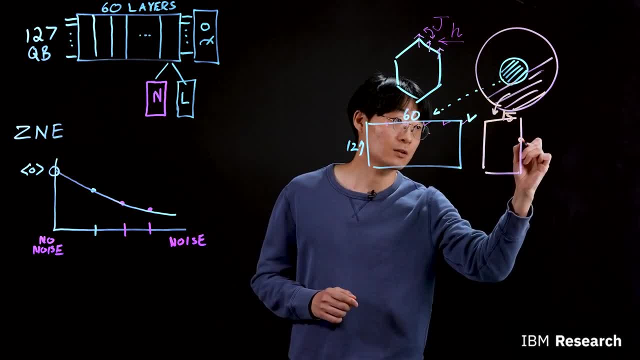 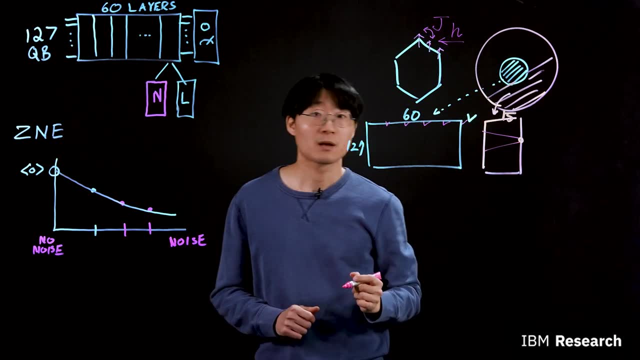 shallower circuit, depth 15, and we examine low-weight observable. In this scenario, we realize that there's a light cone where all the qubits within this light cone really matters for this particular observable. And here's where our collaborator from UC Berkeley comes into play. 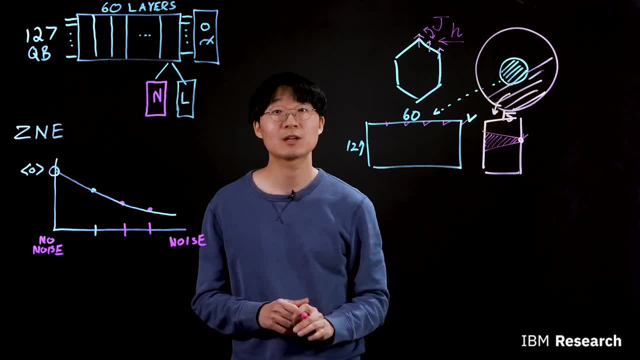 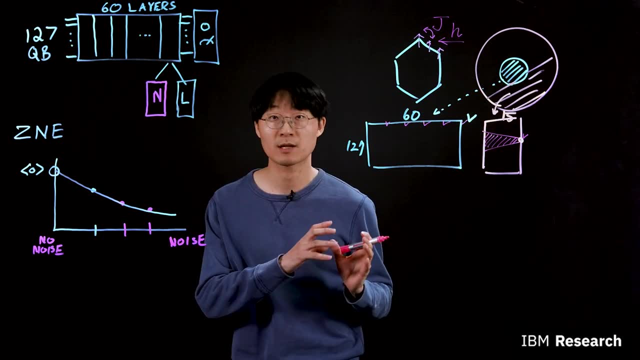 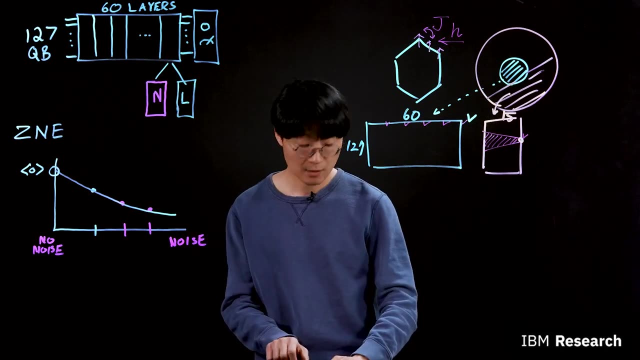 They realize that using the qubits within this light cone, they can use brute force numerics to produce exact solution. So we compare exact solution and our results from quantum hardware and compare against each other. We realize that they have a reasonable agreement. So here's one more check. 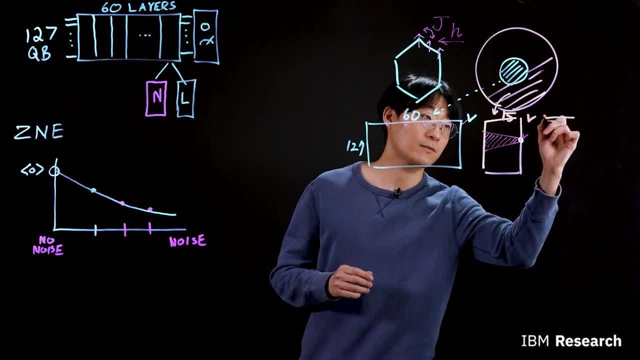 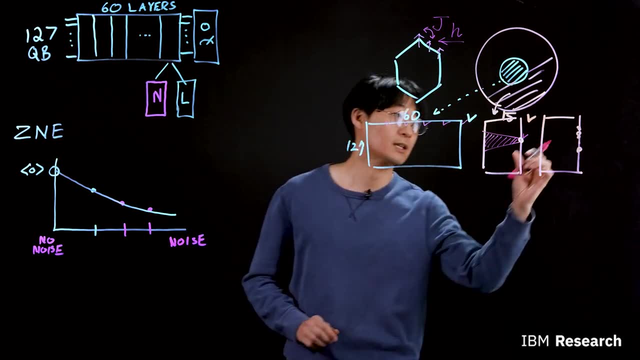 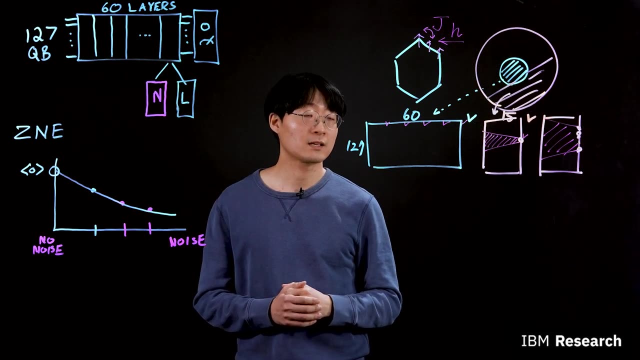 So, with building this confidence, we go one step further. So this time, taking the same circuit, we examine high-weight observable which eventually includes more qubits within its light cone. This time Our collaborators realize that brute force numerics are not feasible. 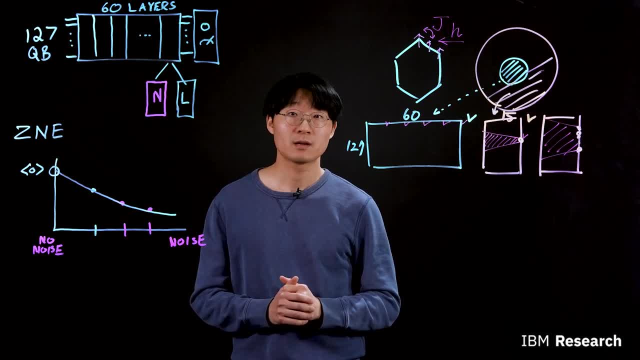 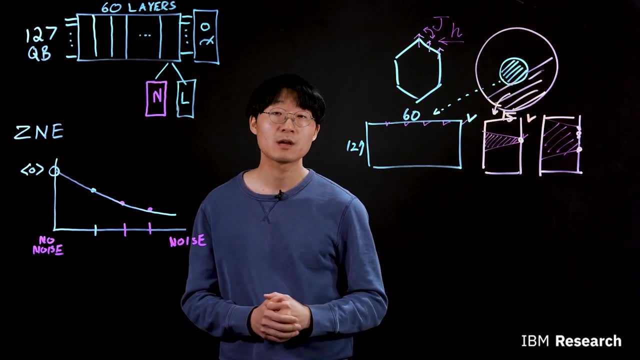 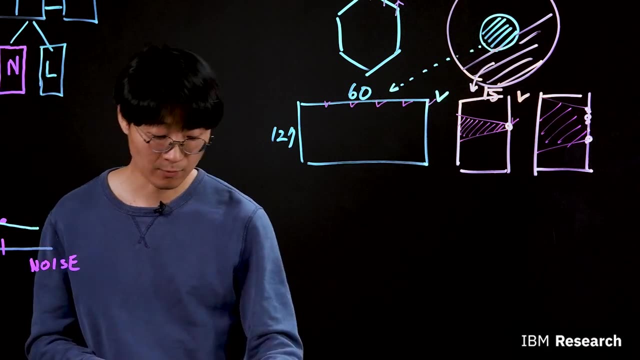 Instead they use numerical approximation method, specifically tensor network method. They realize that using this method they still can obtain exact solution. So we compare their exact solution against our results from quantum computer, And they again agree each other reasonably well. So there's another check. 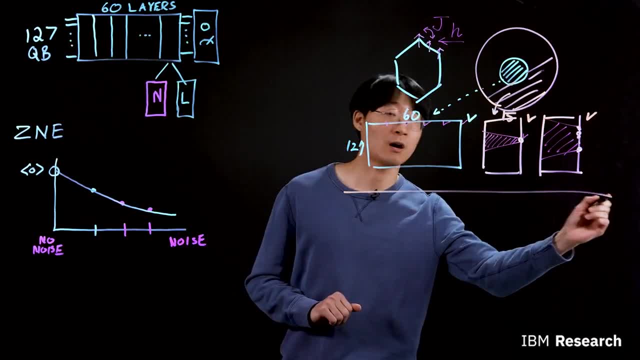 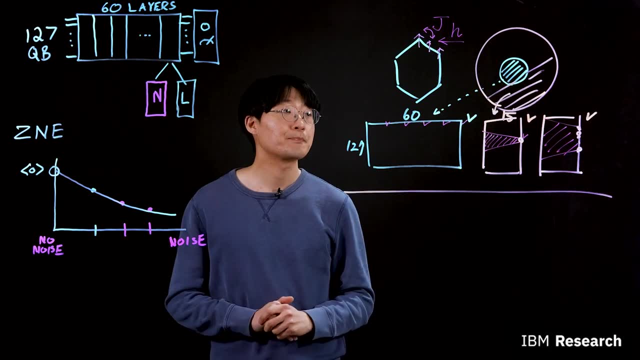 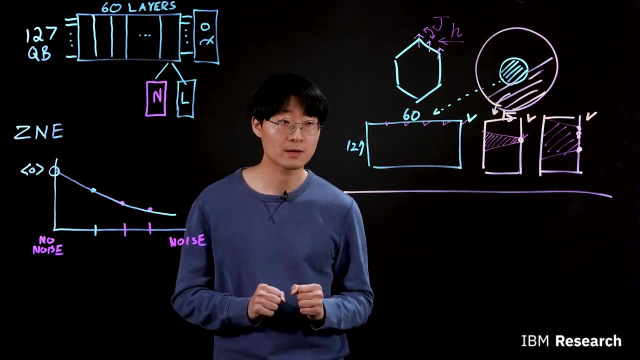 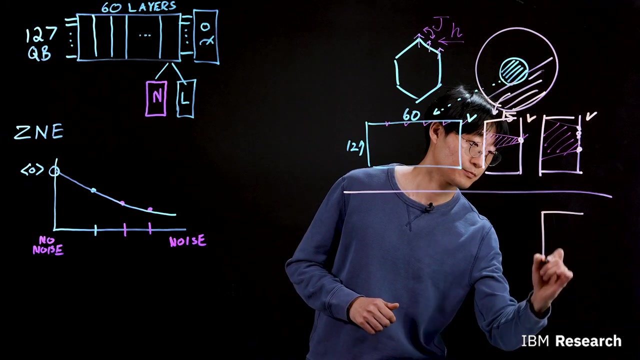 So note that all the results above here are verifiable circuit Meaning. we have exact solution using classical resources. It's crucial step to do this work, to build our confidence on our method. So, as a next step, we would like to go a little bit further, namely, we take the same circuit. 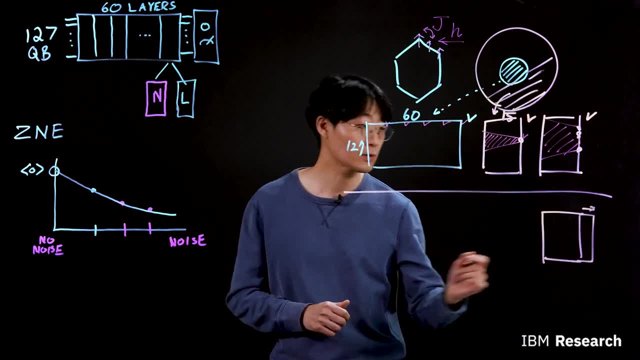 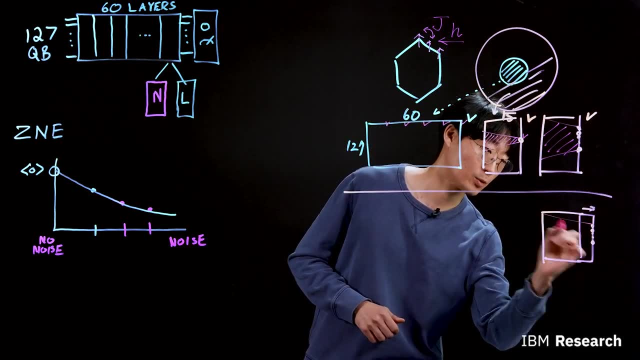 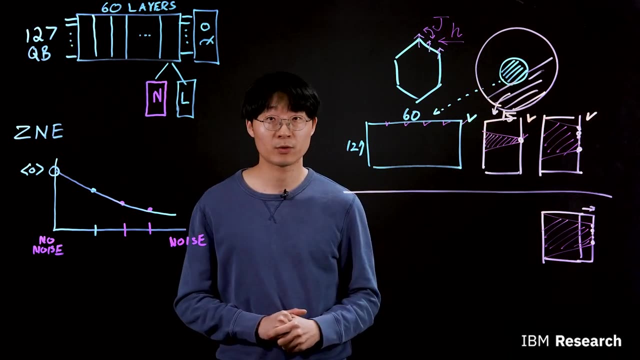 and we progress one more time step to make the circuit a little bit deeper, effectively, And we examine similarly Okay. So in this scenario, our collaborator realized that it's no longer feasible to obtain exact solution even using numerical approximate method. So now we are comparing to approximate solution against our results obtained from our quantum. 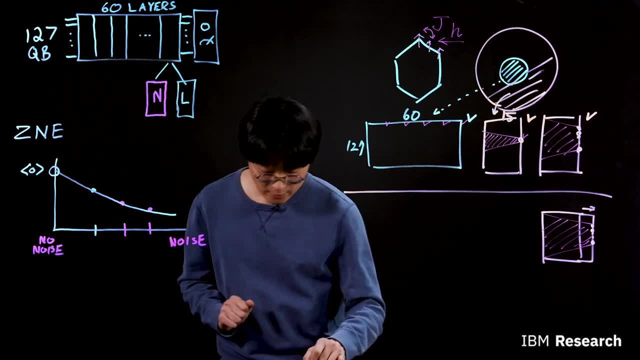 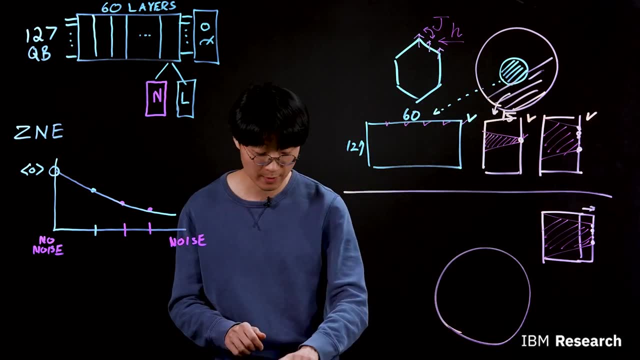 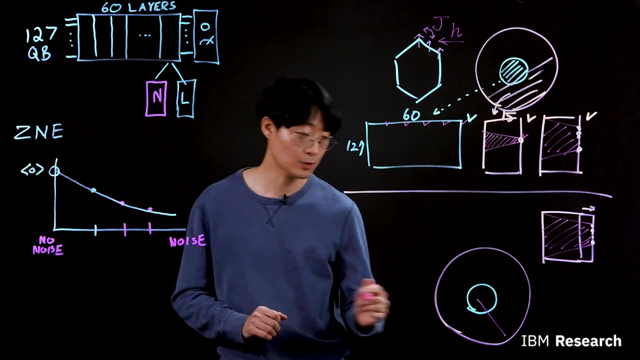 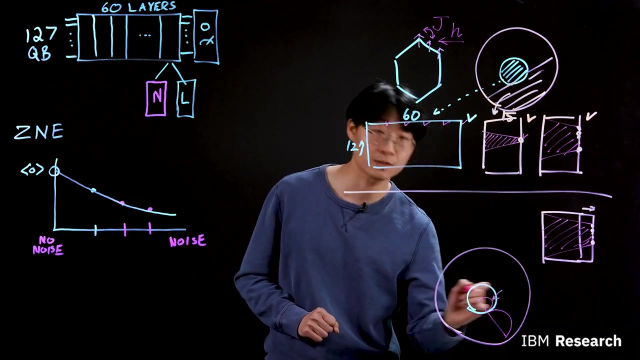 machine. In that scenario, actually, what we ran is following: So again revisiting the parameter space, that results in Clifford circuit here, And we are actually sweeping our parameter that includes non-Clifford circuit as well as Clifford circuit in order to verify our results by looking at Clifford circuit. 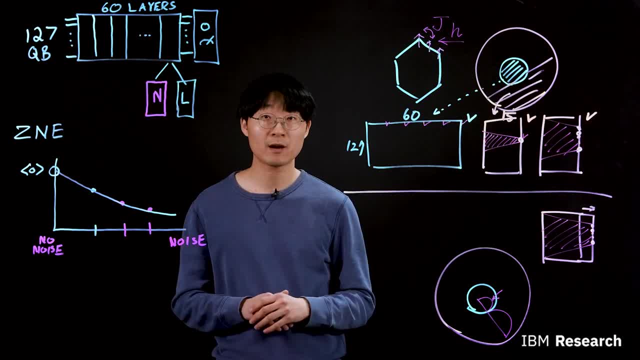 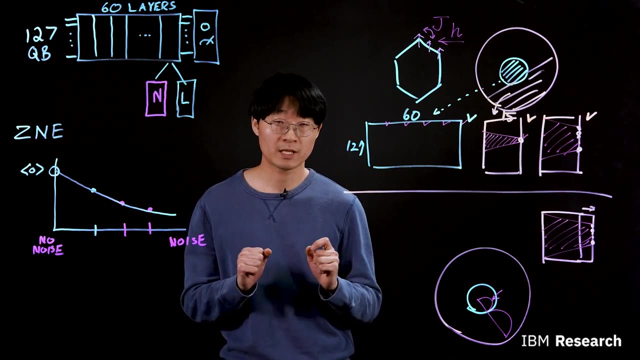 So in this scenario we look at Clifford circuit results and there we see a reasonable agreement between ideal solution and results we get from quantum computer. But for numerical approximation solution from classical computer we start to see some deviation from its ideal value. Of course we don't have exact solution here. 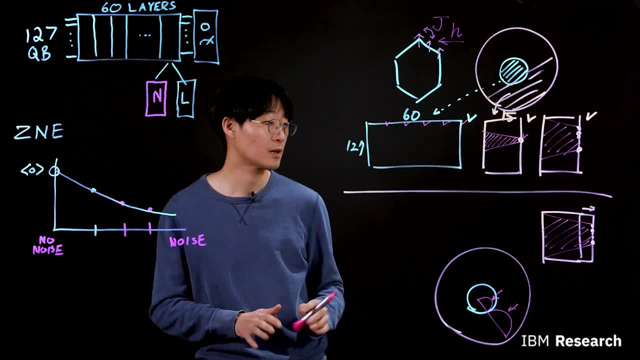 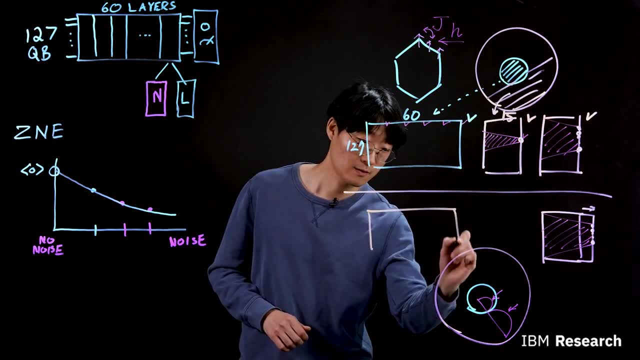 So any results from non-Clifford circuit represents unverifiable circuit. So we need this. we need the same practice, very similar practice, but this time we go all the way to all the way to depth 60. And we look at low-weight observable. 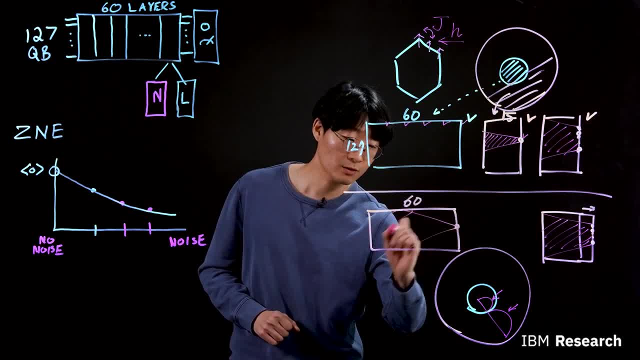 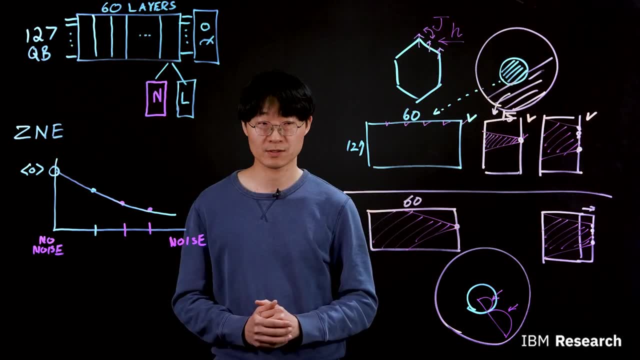 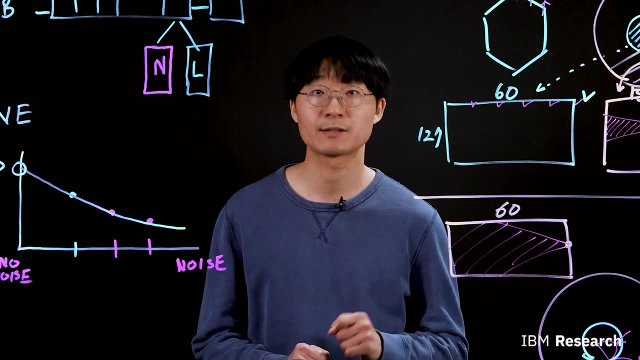 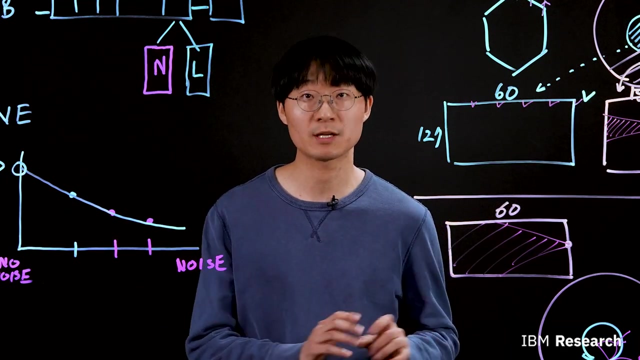 Okay, Which eventually covers all the qubits within this light cone, And we observe very similar behavior that produces reasonable but unverifiable results. Looking ahead, we believe that some researchers will find a way to verify our currently unverifiable circuit. That's good, because it means quantum is driving an innovation to classical computing. 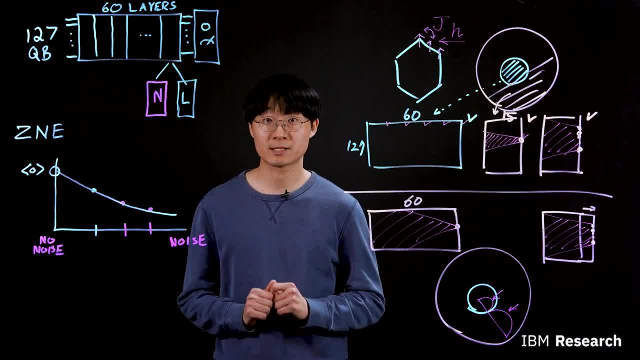 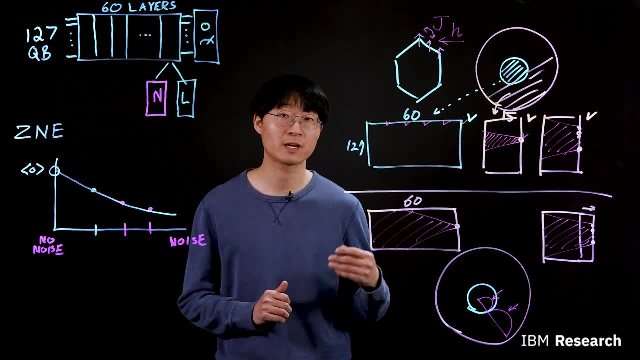 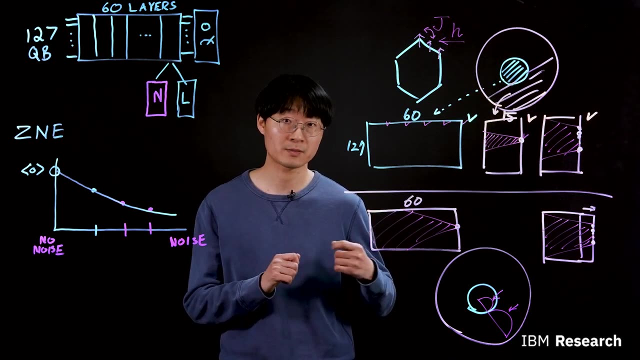 Using their technique. if they prove that our results are reasonable, that's again good, because it means noisy quantum computer can produce reliable estimate on observable of interest. And of course, as hardware innovation progress and our hardware gets better and better, we'll have further access to deeper and larger circuit. 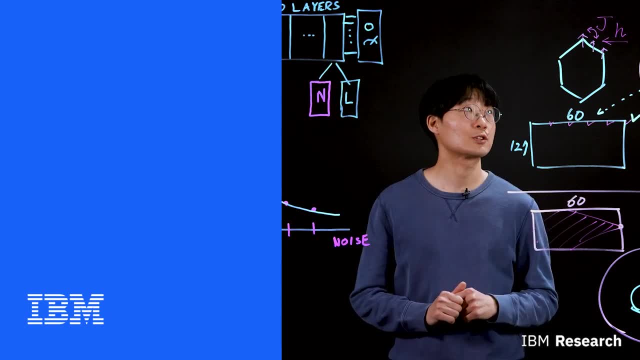 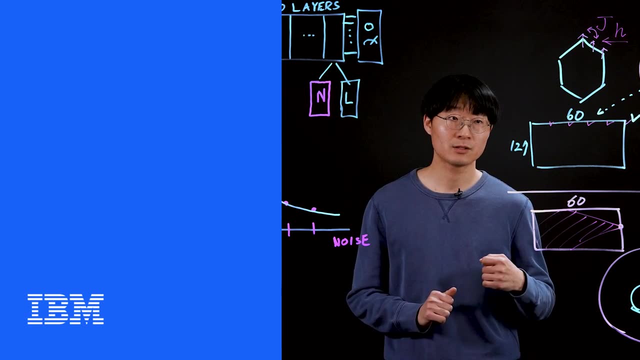 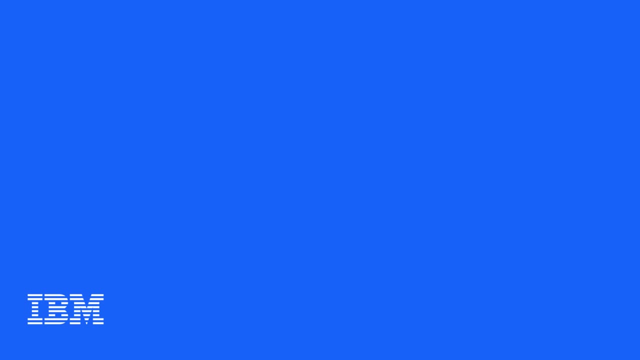 And we believe that this type of research eventually bring us one step closer to a day when a quantum computer can tackle truly useful problem. I hope you like this video. Be sure to like and share this video. Thank you for your time.